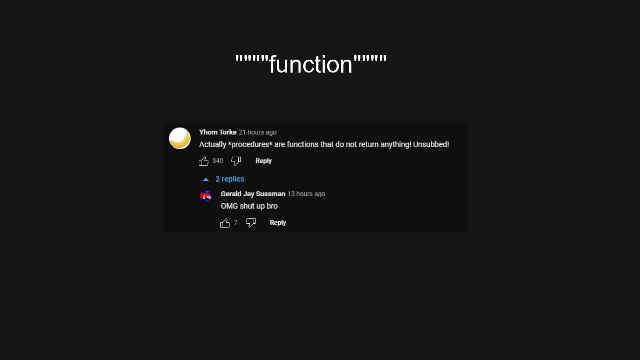 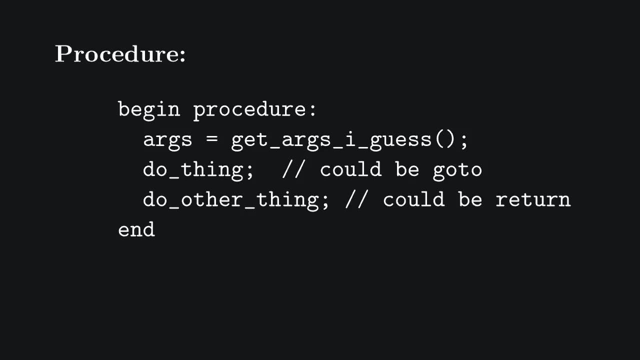 as opposed to a function which does In this video. by procedure I mean any sequence of instructions which may well contain a return, while a function in the functional programming sense is a much more abstract idea which may well contain a return. 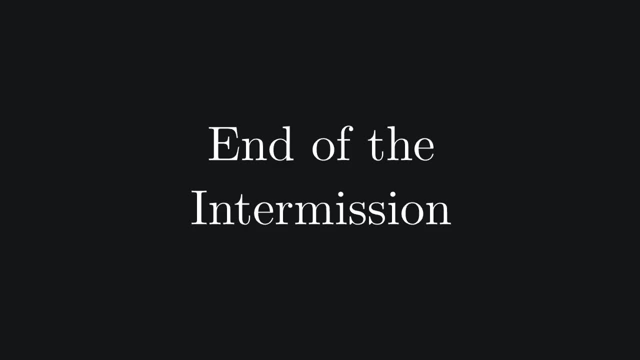 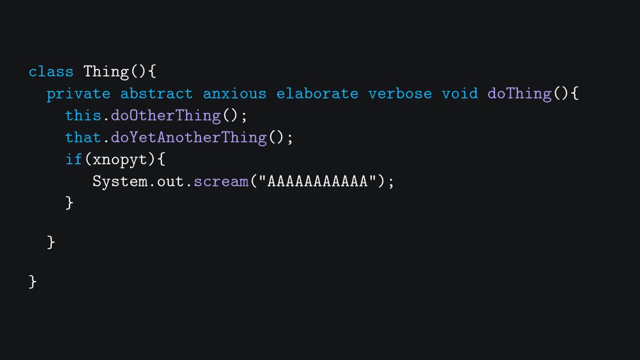 Which we will explore later in the video. Java and its classy friends, on the other hand, are called object-oriented languages, but the instructions inside their methods are still commands, so these languages are still based on the same imperative paradigm, One of the things that make functional languages most different. 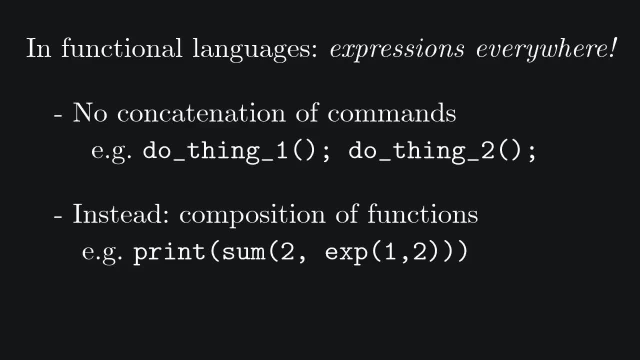 from the ones you're probably used to is the fact that the instructions are not commands but expressions, and a program is not a concatenation. A program is not a concatenation of declarations and commands, but a composition of functions. We'll call this property 1.. 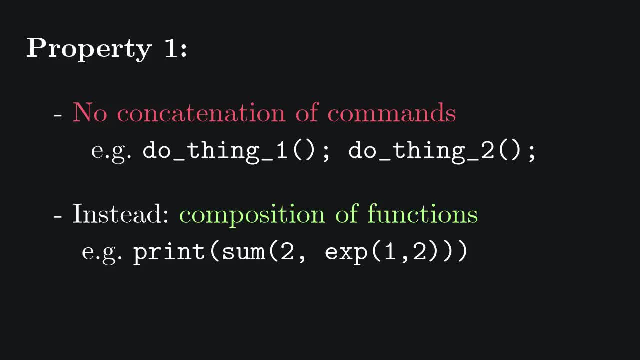 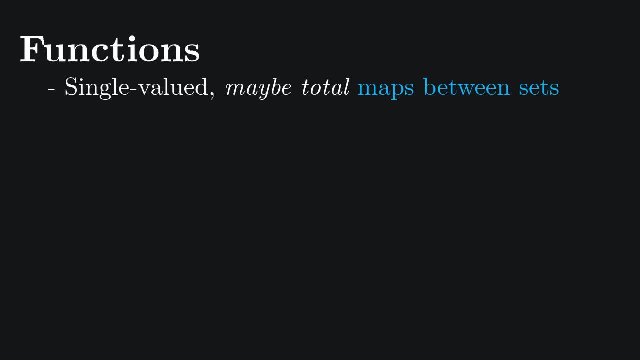 There's also another big difference, the biggest one probably, and I'll introduce it later in the video. When we refer to functions, we mean it in the mathematical sense of maps between sets, such that the output depends solely on the input. A procedure can be a function. 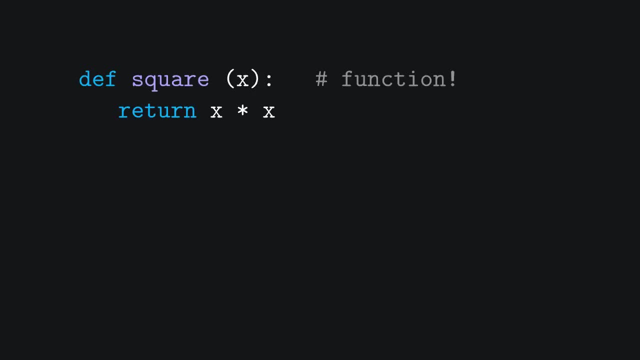 for example, this Python procedure is a function that takes an integer and returns an integer. In mathematical notation we would write this function as f from integers to integers such that x maps to x squared. This symbol here means maps to and writing f such that x maps to x squared. 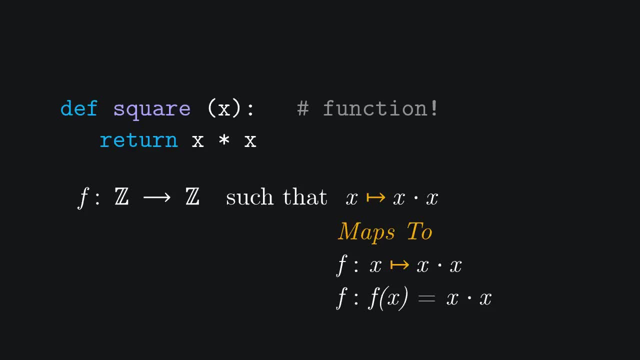 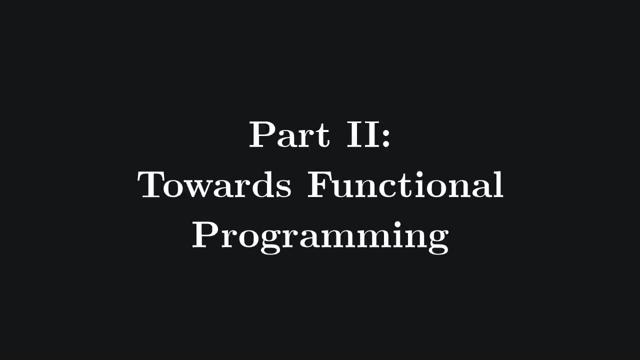 is equivalent to writing f, such that f of x equals x squared. I prefer to use the maps to notation here, since it allows for a better transition. later in the video Let's look at another example that should bring us a little bit closer to the functional paradigm. 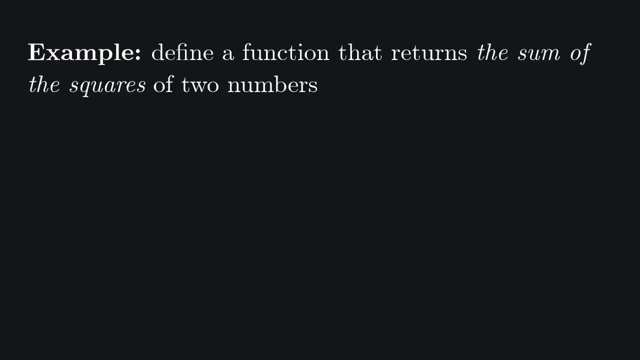 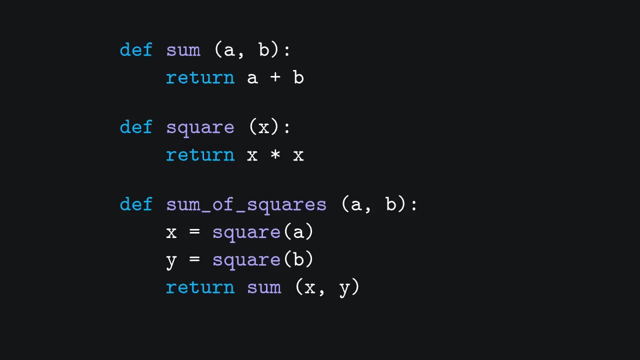 If we wanted to define a Python function that returns the sum of the squares of two numbers, we could either write the following procedure or, if we wanted to separate the operations, write something like this: Now remember what we said about the functional paradigm. 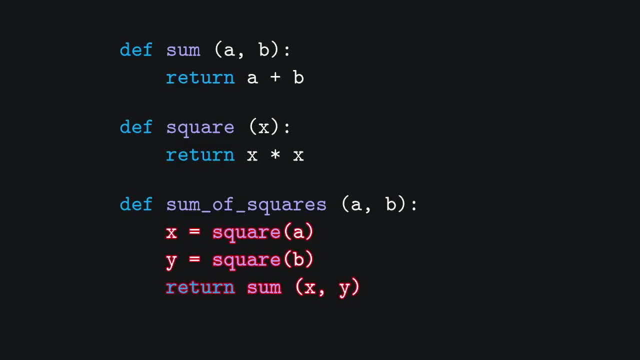 property 1.. Rather than using a concatenation of declarations and commands, we want to use function composition so we can rewrite the function like this. This is closer to satisfying the first property. There is still a problem though That return thing over. there is a command. 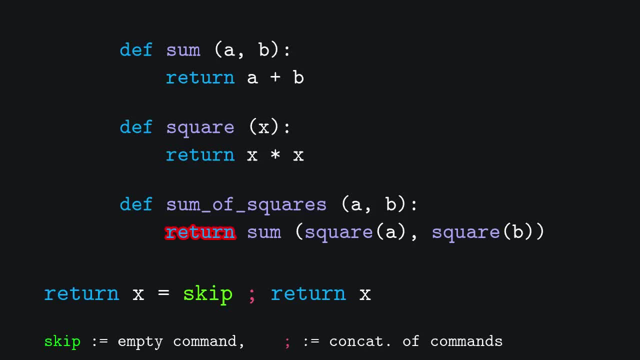 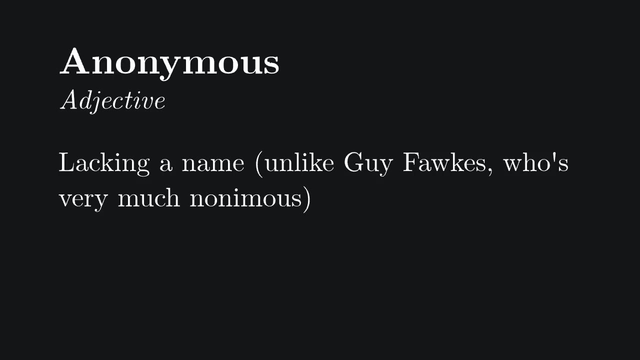 and one command is enough to make this computation a concatenation of commands, thus violating property 1.. We can solve this by introducing a second property of functional programming languages: the presence of anonymous functions. An anonymous function is a function without a name. 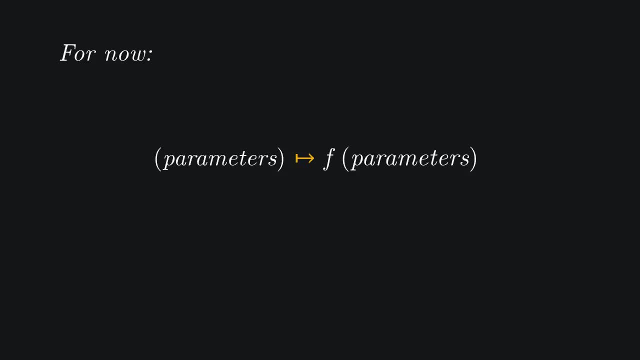 We will represent anonymous functions, at least for now, by means of the maps to notation, Instead of writing our function like this. we will stop using Python for a while and represent our function in a weird mathematical pseudolanguage like this: Notice that we use the same equals symbol. 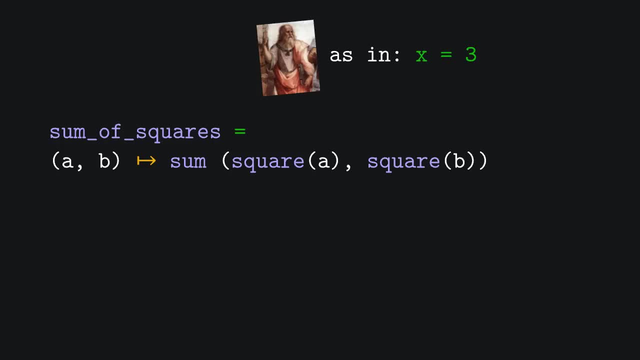 that we might have used to assign the value 3 to an integer variable, x. This is a hint to the most important property of all. Anonymous functions can be assigned to variables the very same way that a number can be assigned to a variable. 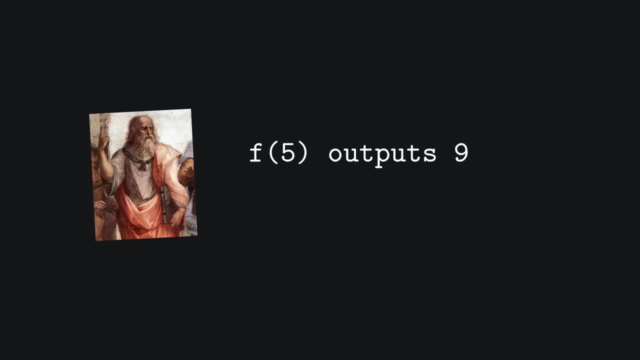 Numbers can be the inputs and outputs of functions. so I guess the next obvious step would be using anonymous functions as the input of other functions like so, and also as the result of other functions. In this case, the function foo is a function. 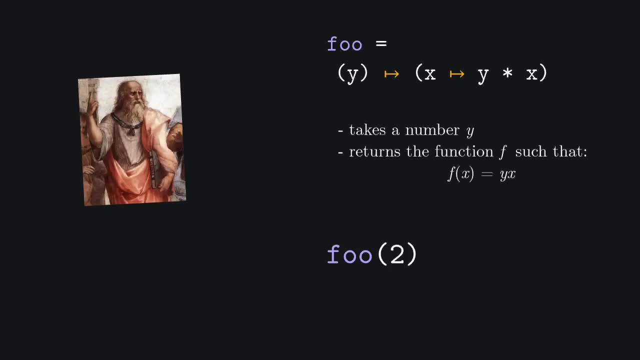 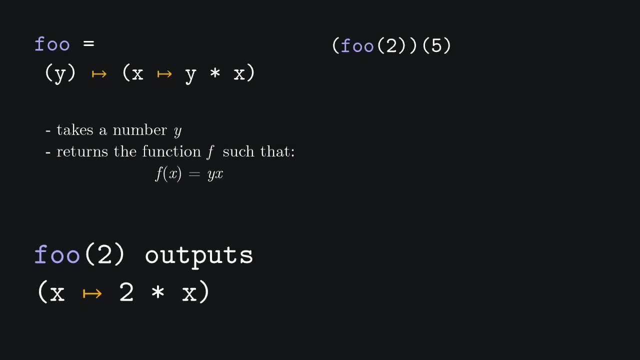 that returns a function. so this returns the function that multiplies the input by 2. Hence the following: computes the value 2 times 5.. Should we call this property 3? I guess This is, I think, the most important property. 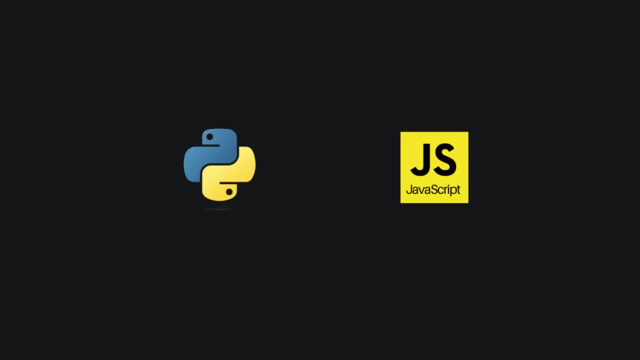 of functional programming languages. This may or may not surprise you, but several languages you may already know, like Python and JavaScript, already have the possibility of writing programs that satisfy these three properties. For example, you can write anonymous functions and pass them to other functions in Python. 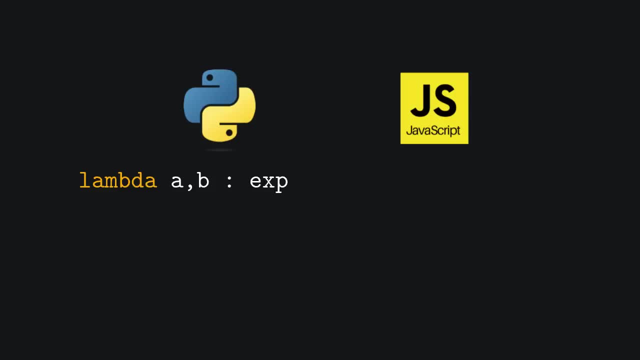 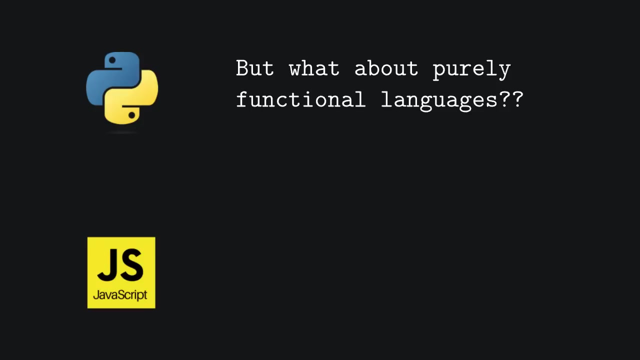 by using this syntax and, in JavaScript, by using this other syntax. This is because these languages are multi-paradigm languages. But what about purely functional languages? Python and JavaScript allow us to use functional tools while still having the possibility to concatenate commands. 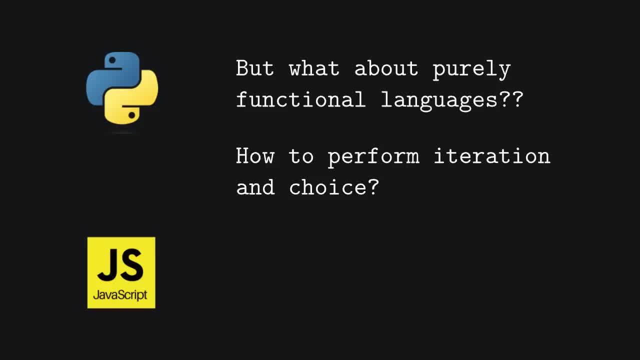 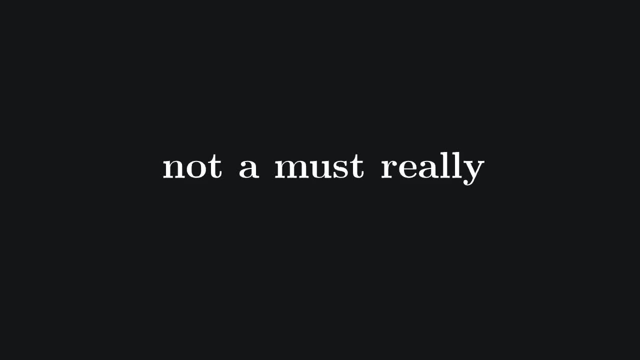 How do you do, like iteration, without the ability to concatenate commands? In purely functional languages we don't have iteration, but it's not really necessary. Functional languages use recursion as their equivalent of iteration. As you may know, every while loop can be transformed. 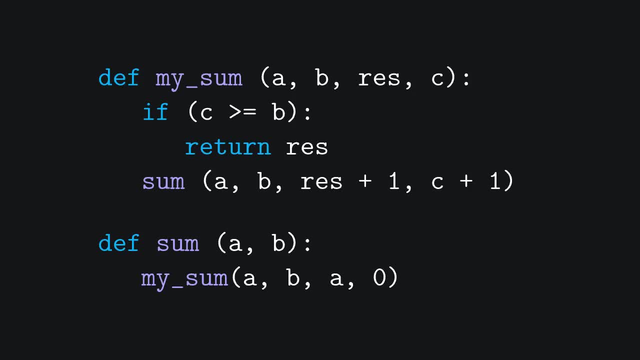 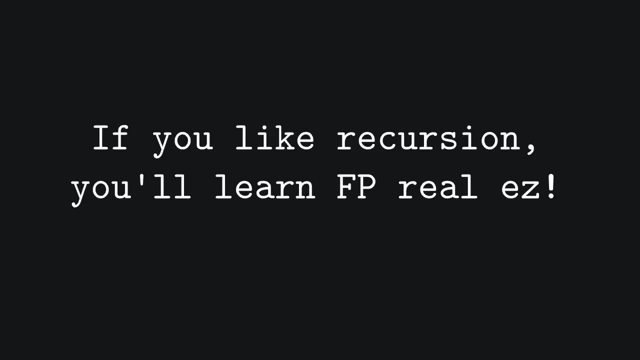 into a tail recursive function by moving the variables you're checking from the guard to the base case of the recursive function. If you're familiar with recursion and you're using it already in your paradigm of choice, the transition to any functional language will be quite smooth. 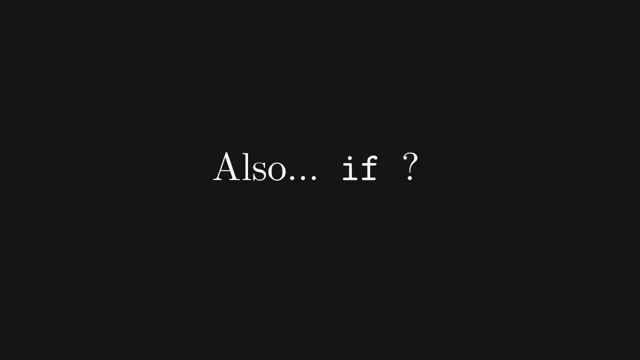 Another thing you may be asking yourself is: what about conditionals? Well, I'm sure you've used some sort of inline conditional already, or ternary operator, so it's basically the same, And this is already most of what you need to know. 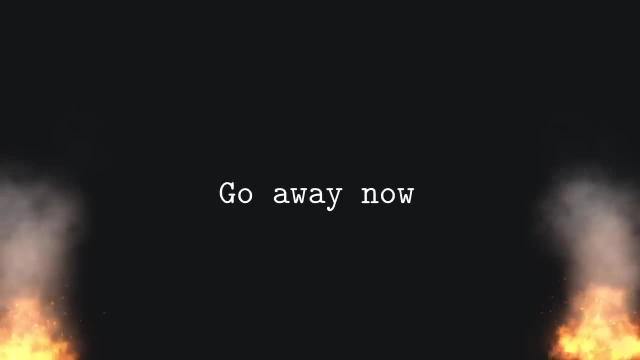 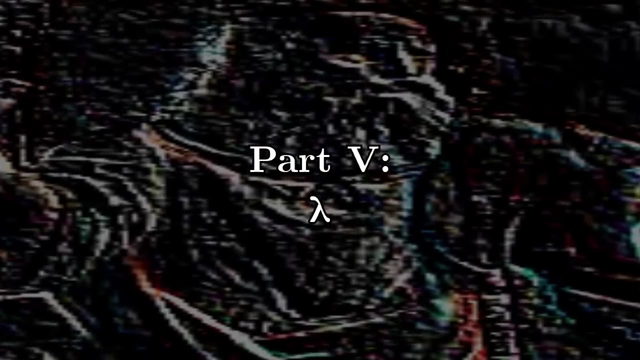 in order to have a vague idea of what functional programming is like. But you want the good stuff, don't you? The lambda-juice, the code, the purity, the platonic world of ideas. The Python syntax for anonymous functions contains the word lambda. 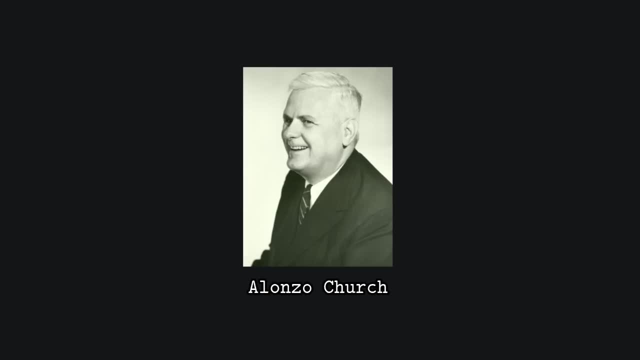 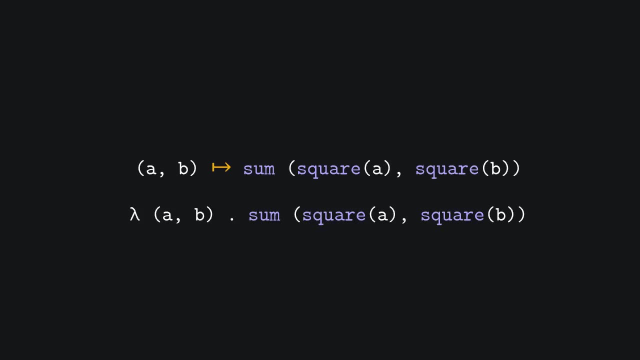 This is derived from a notation introduced by Alan Turing's color friend, Alonzo Church. He wrote the functions I represented with a maps2 with a different notation that features the Greek letter lambda. Actually this is a bit wrong, since in lambda calculus 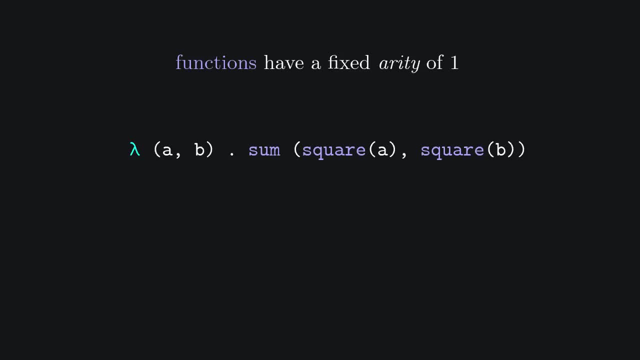 which is what we're doing right now. functions have a fixed arity of 1, which means they only have one parameter. Functions with more than one parameter can be simulated by doing something like this If the previous function was, in mathematical notation, a function from the integers. 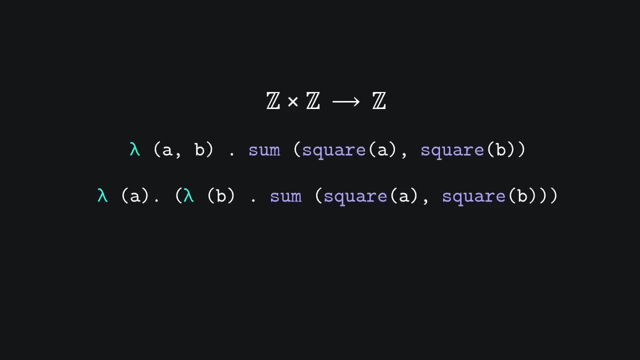 times the integers to the integers, which means a function that takes couples of integers as its input and returns a single integer. this new function is from the integers to the set of functions, from the integers to the integers. It is quite simple to show that these two functions 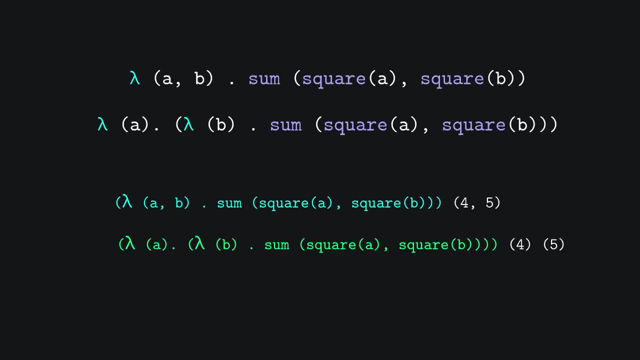 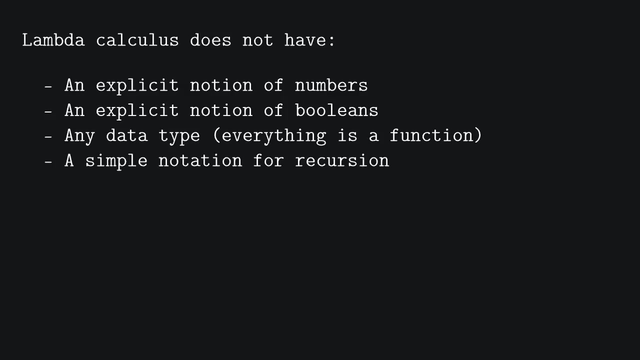 called in these two different ways are, in fact, equivalent. This property is known as currying. To be even more precise, lambda calculus does not even have an explicit notion of numbers or operations, or Booleans or even recursion, For example. 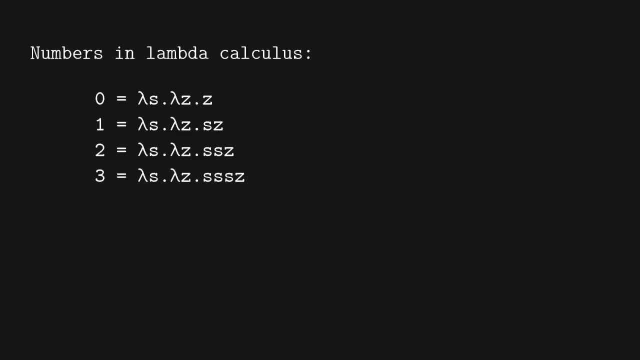 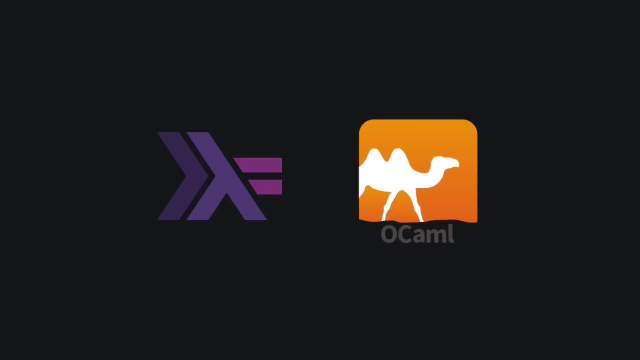 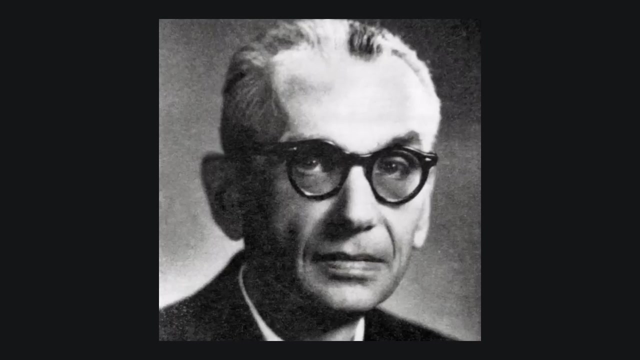 numbers are represented like this, And this thing called the y-combinator makes recursion. Luckily for us, we don't need to use the lambda calculus in its original form, just like we don't need to use Turing machines or general recursive functions. 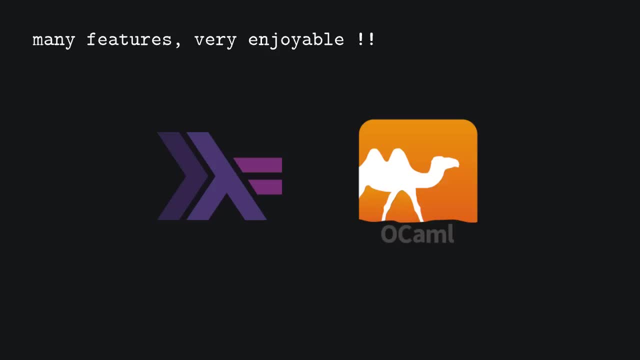 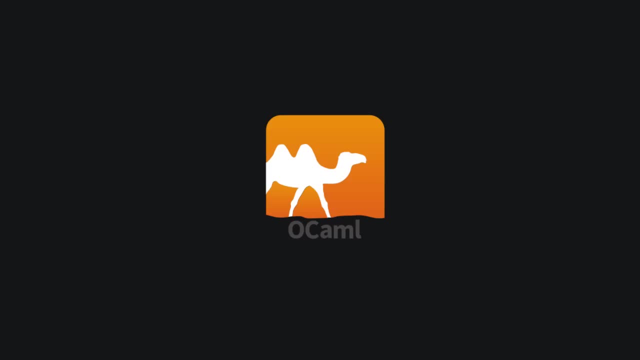 In fact, modern functional languages are very rich of features that make them very suitable for some tasks. The functional language I'm most familiar with happens to be OCaml. The most powerful tool in OCaml is one called pattern matching, The simplest way I can describe 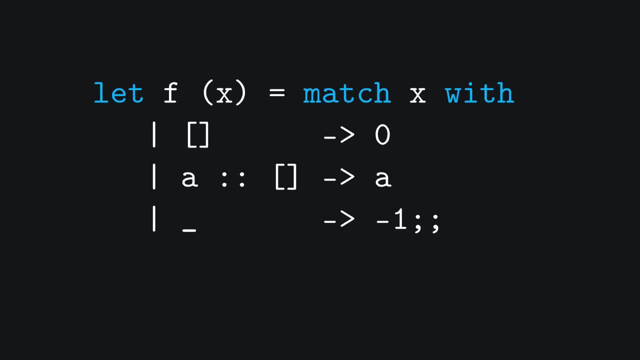 pattern matching is. it's like a switch, but rather than checking the value of a variable, it checks whether an expression matches a pattern. This, used together with algebraic data types, makes writing interpreters in OCaml almost trivial. A lot of verification tools. 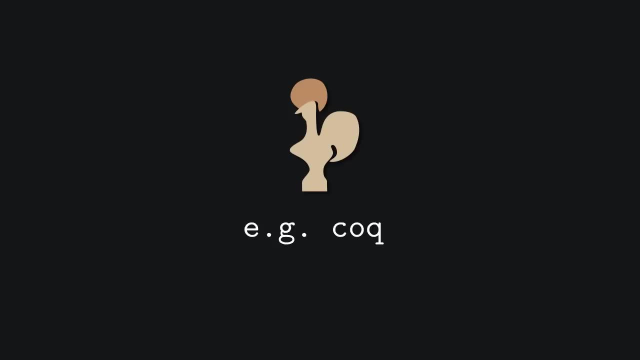 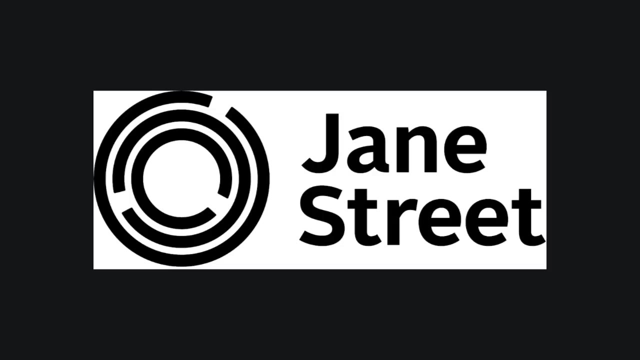 and proof assistants are based on functional programming and some of them are written in OCaml. Apparently, there is also at least one company that uses OCaml for their services. But why am I saying all this? Why do I have to point out 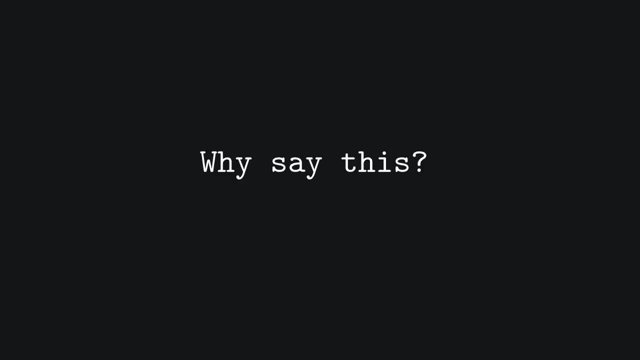 that there actually are areas in which functional programming is much more suitable than other paradigms. Well, because you may have heard some people claim that ha, functional programming is useless. I mean, computation without states is sure elegant, but no collateral effects. 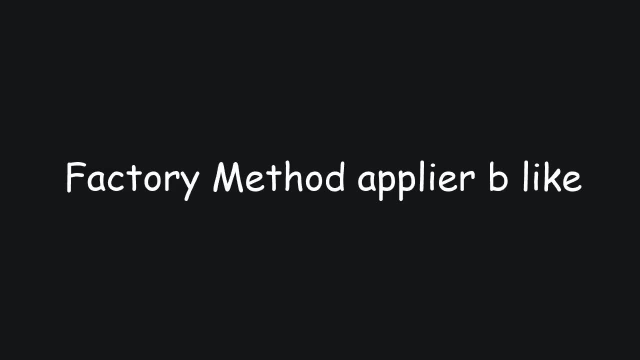 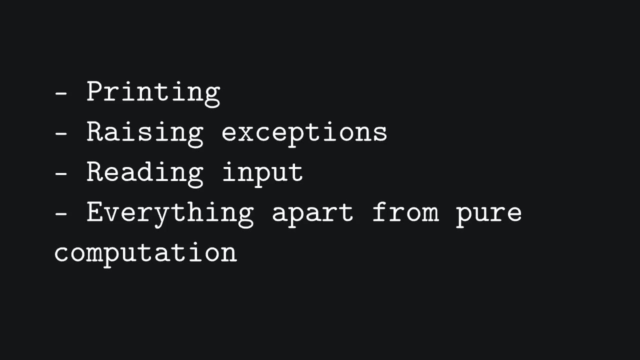 How can a programming language be useful if it can't even print a screen? So apparently there is one thing I forgot to mention: Collateral effect. If you cannot concatenate commands, you cannot do something like this: Printing, raising exceptions and other things like these.